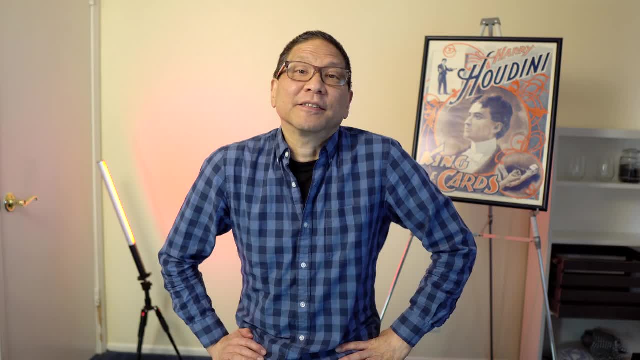 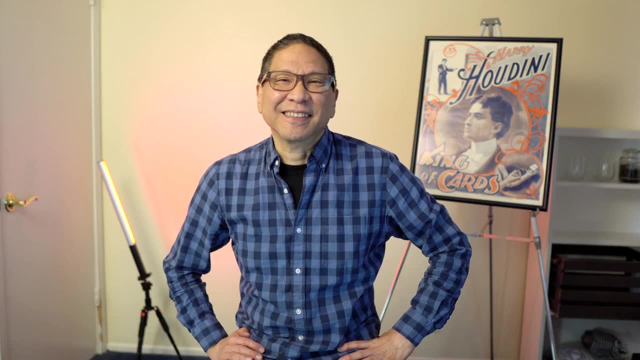 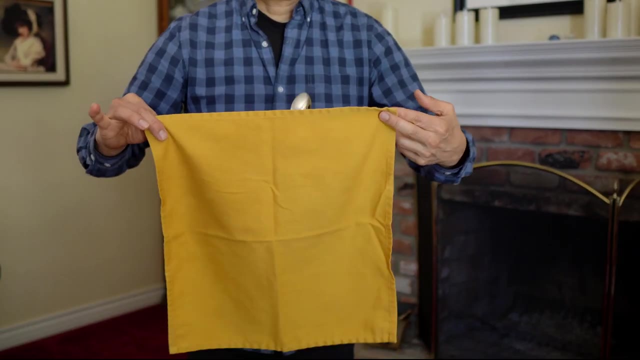 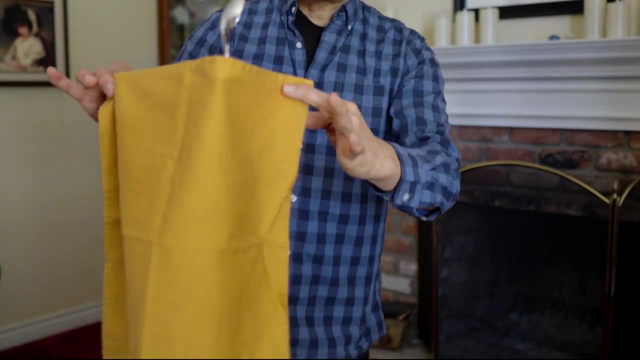 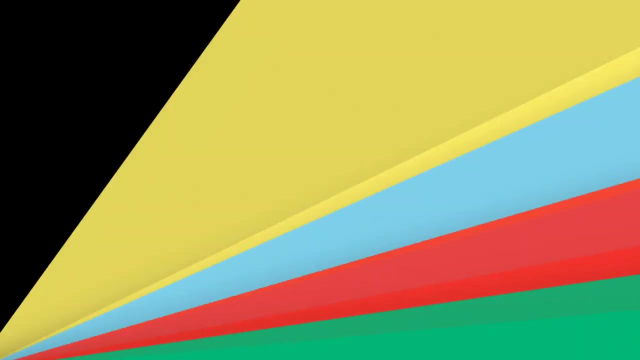 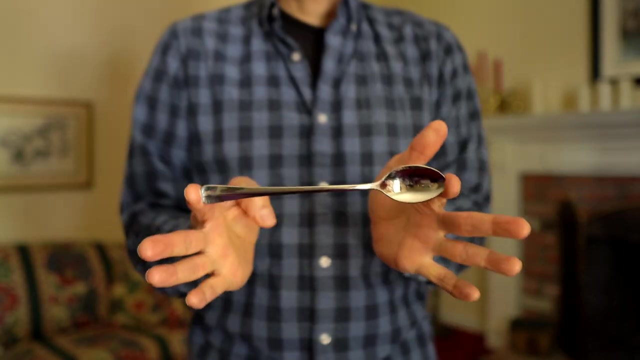 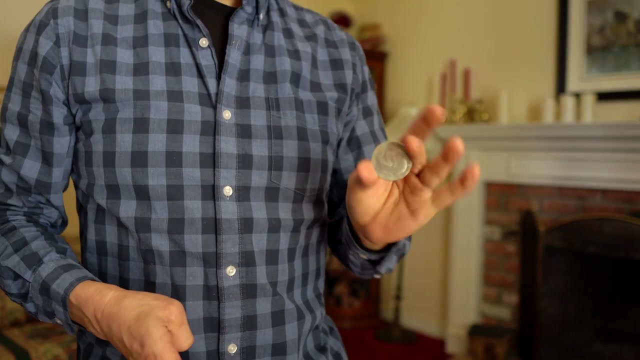 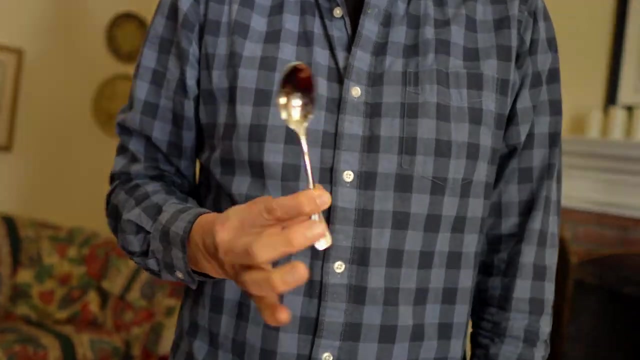 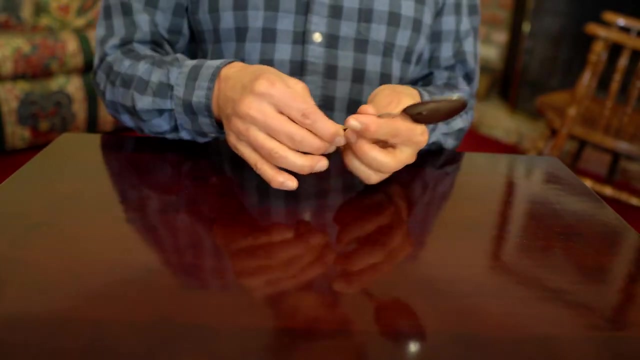 You're about to learn three ways to bend a spoon, as well as a host of easy magic tricks that employ spoons. First I'm going to show you the tricks, and then I'll show you how to do them. Let's get started. Let's get started. 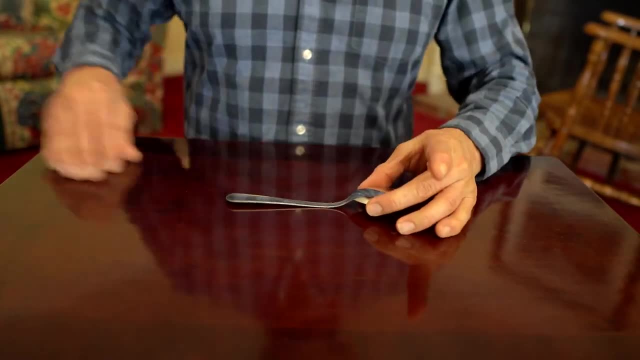 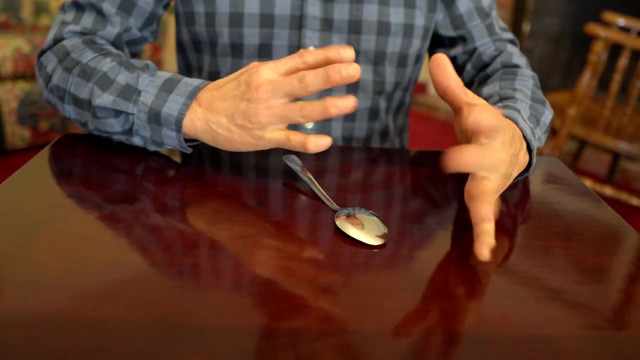 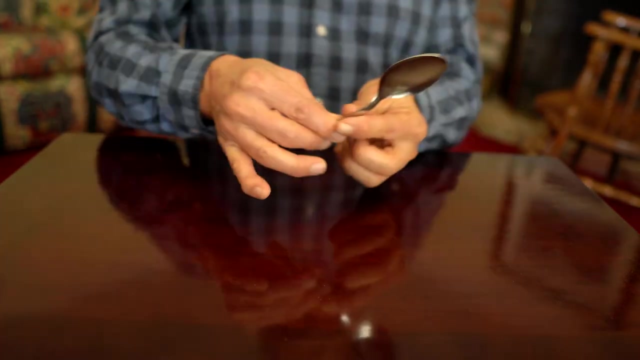 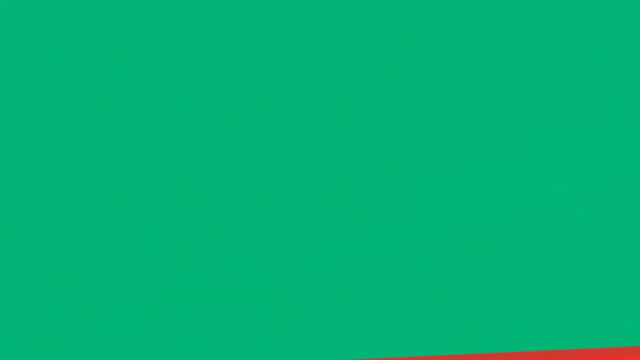 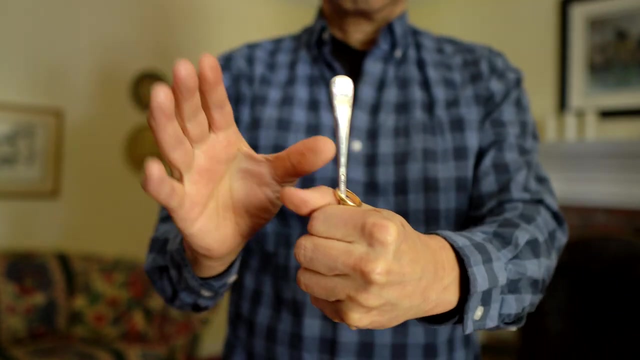 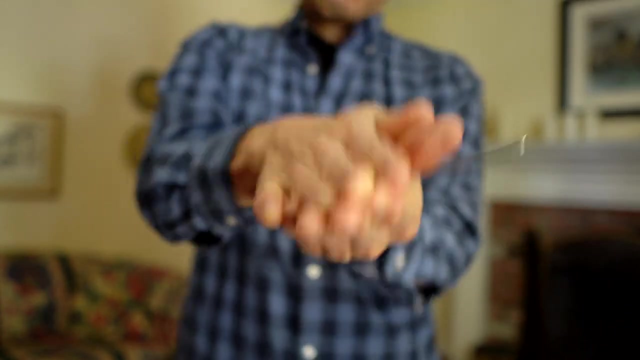 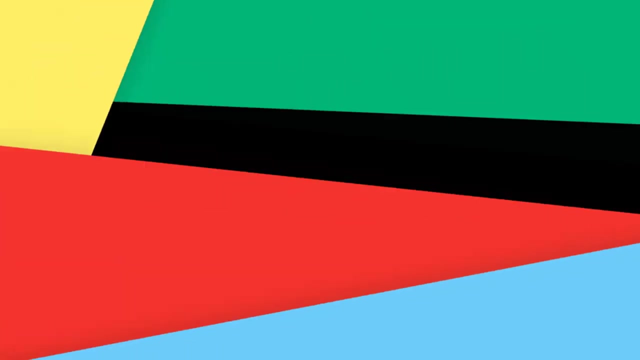 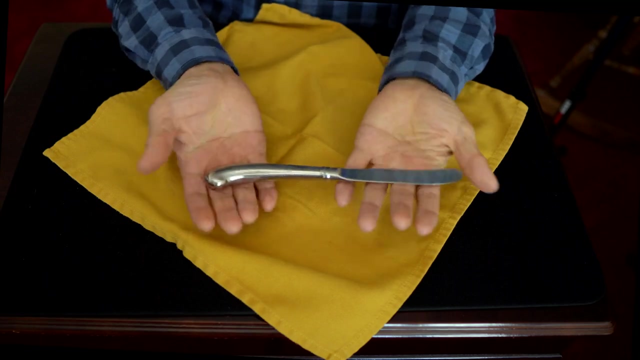 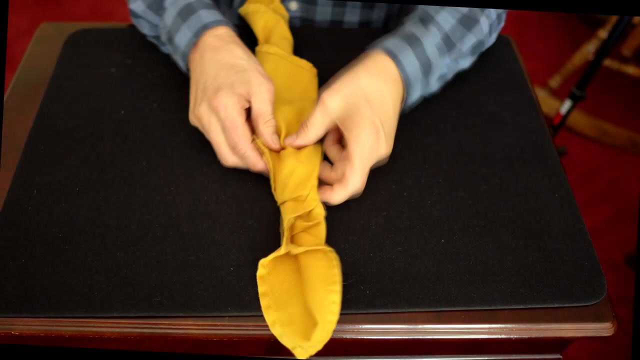 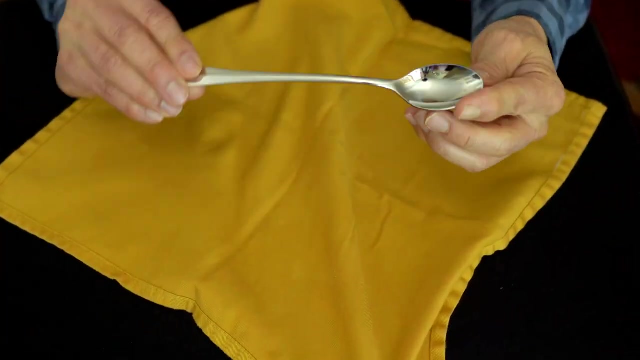 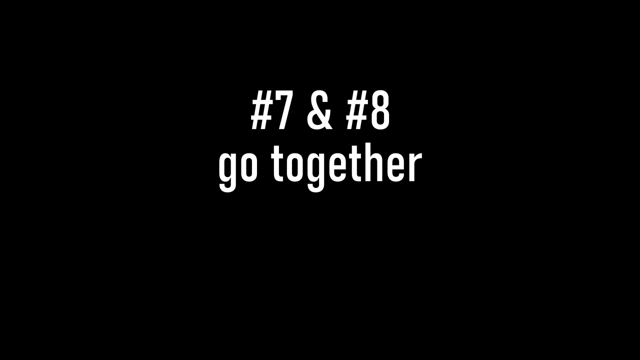 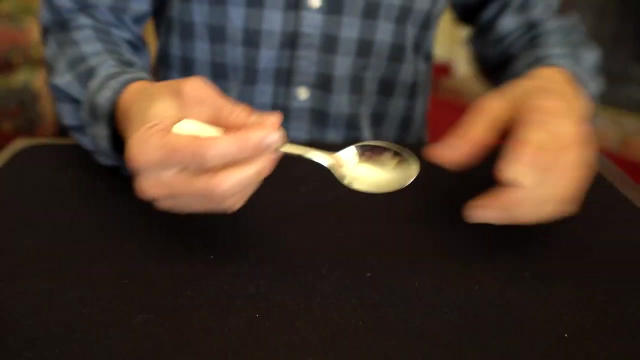 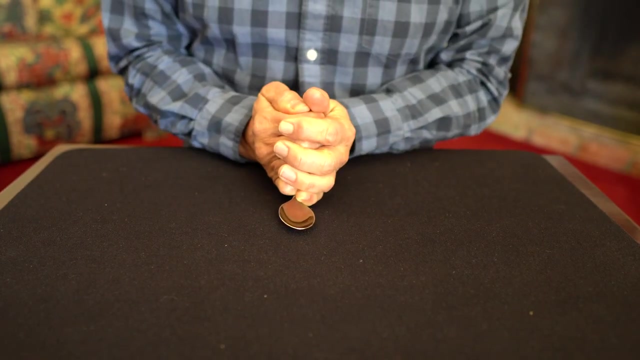 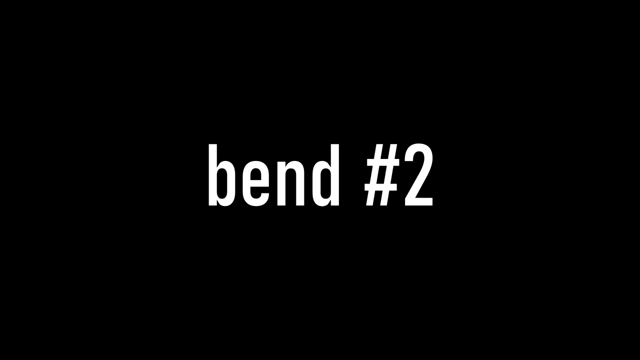 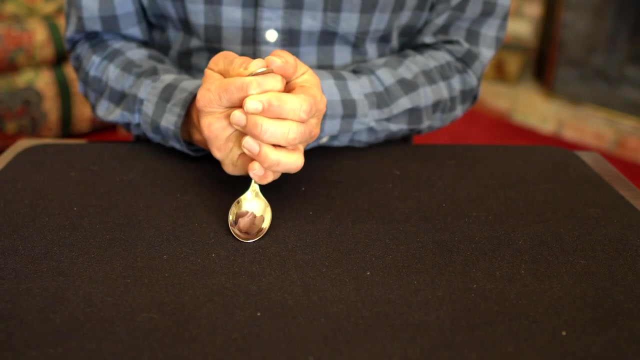 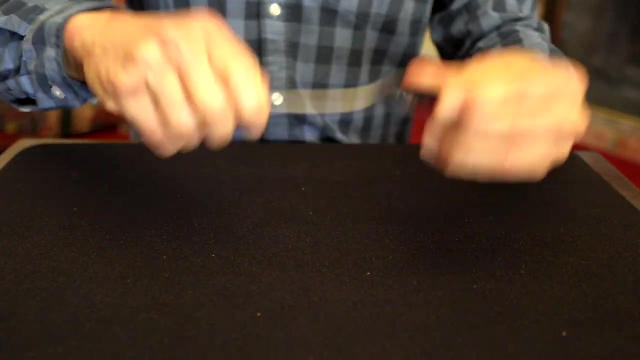 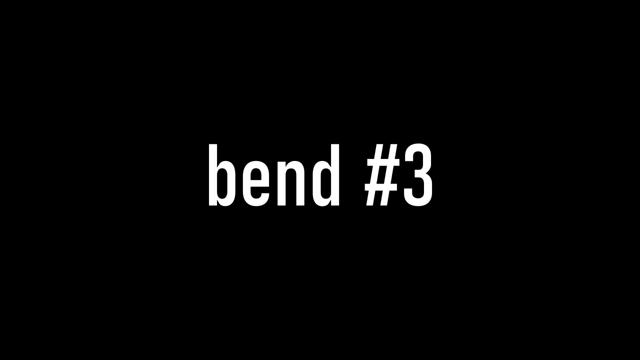 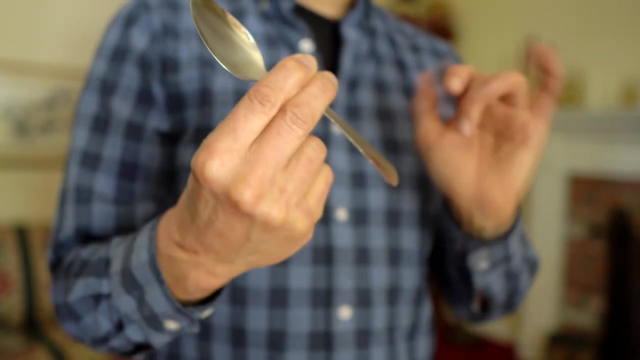 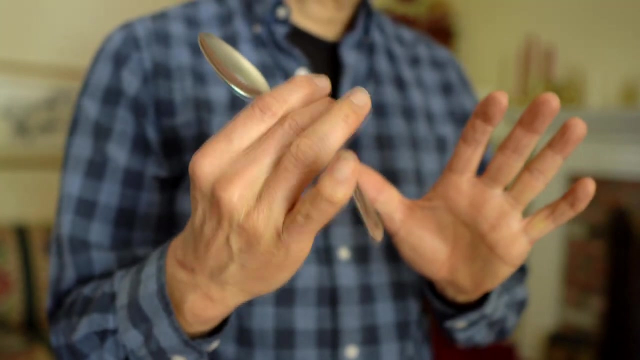 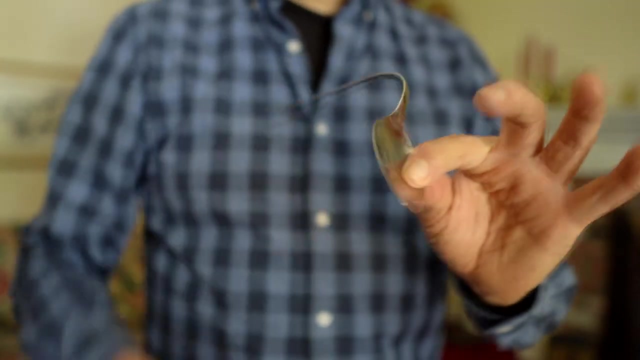 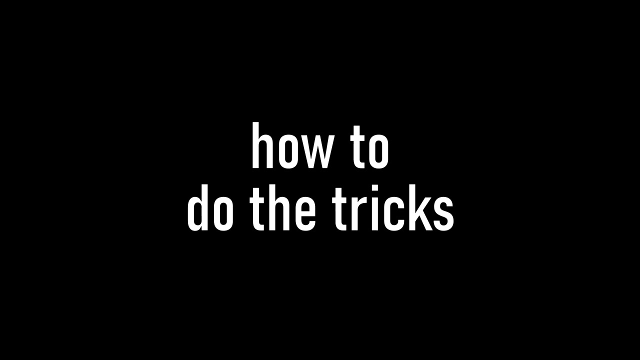 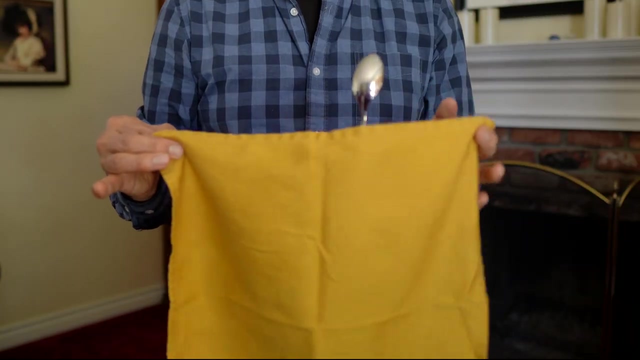 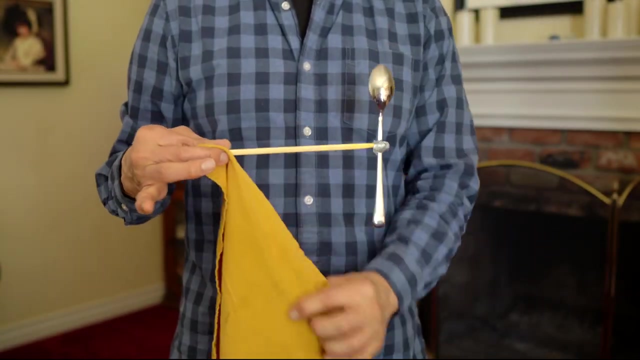 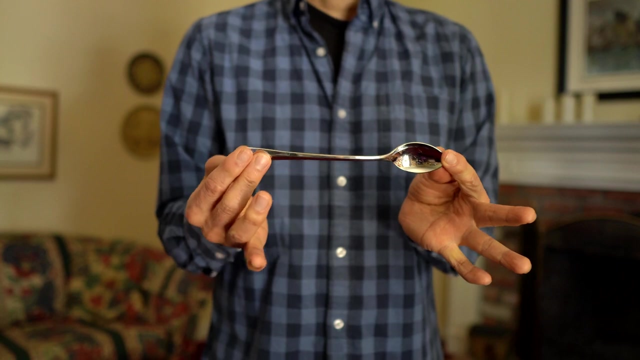 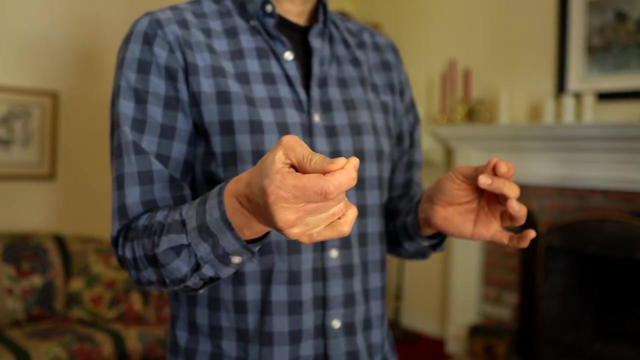 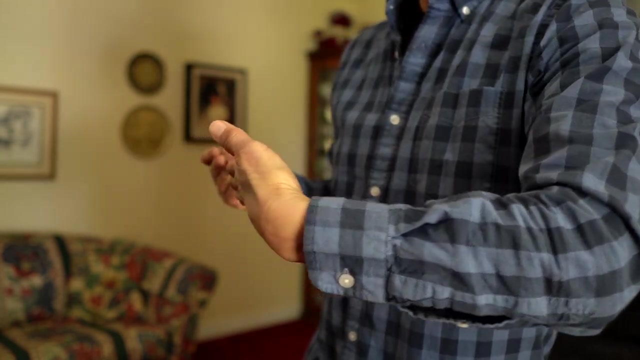 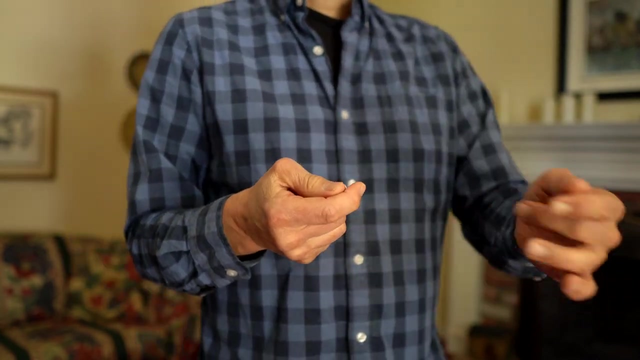 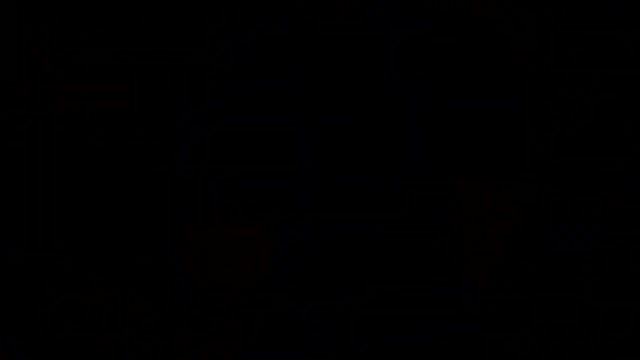 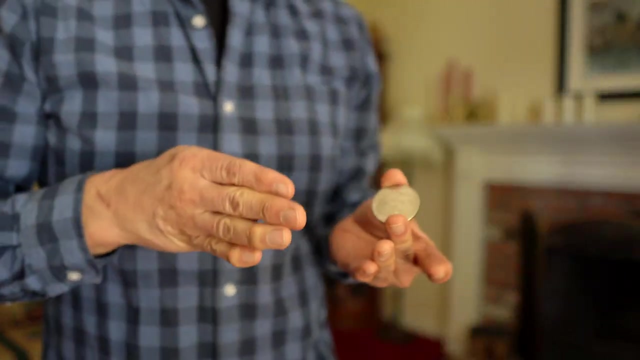 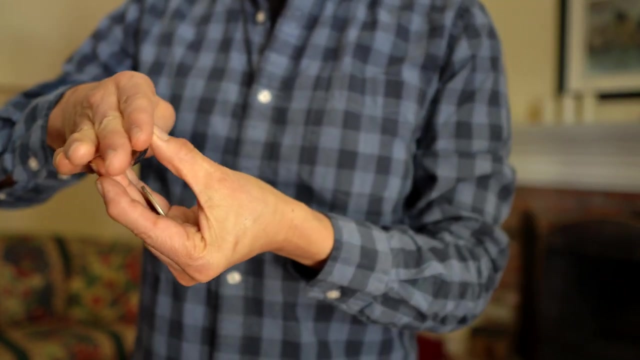 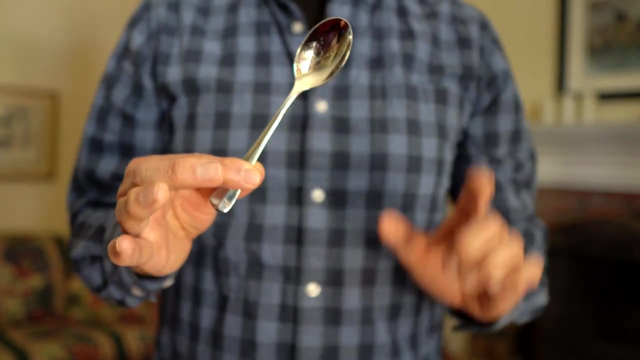 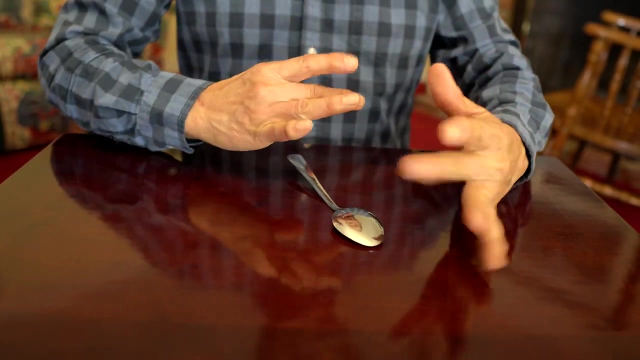 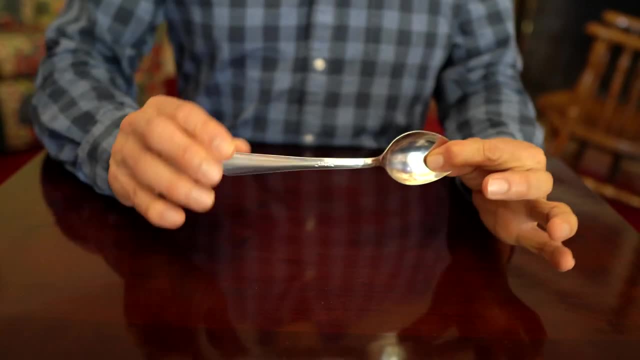 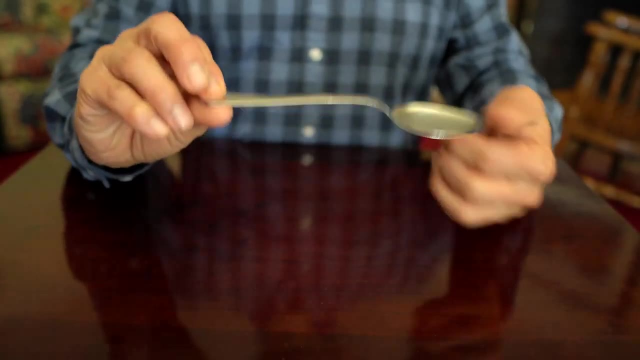 better because it's magnetic, because in your hand over here, I have a band-aid and a magnet here taped on the hand, and that is the secret. So take your very inexpensive spoon. You're gonna have to bend it a little bit. You're gonna have to bend it a little bit. You're gonna have to bend it a little bit. 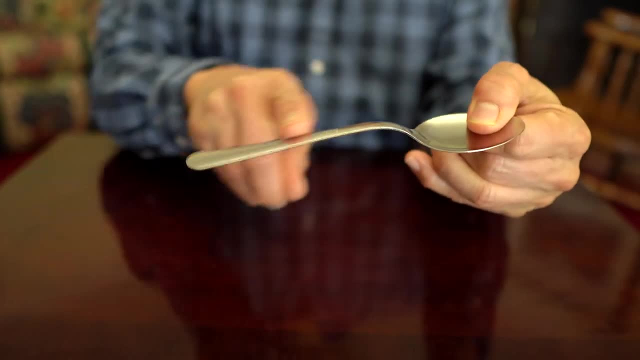 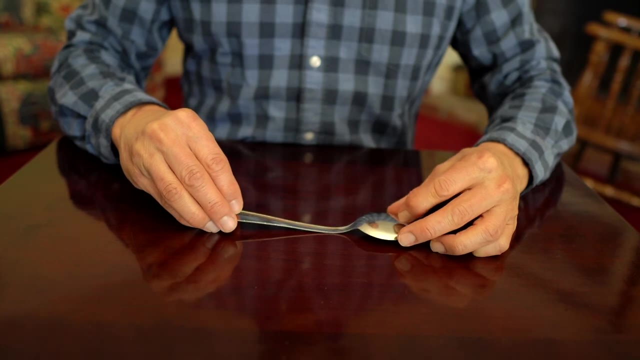 You can notice that the profile is a little off here And that's because I made it so there's a little bit of a balance point here and that way it balances and will freely turn. So all you do is bring your spoon out and into the weight of your hand and really make sure it's balanced. 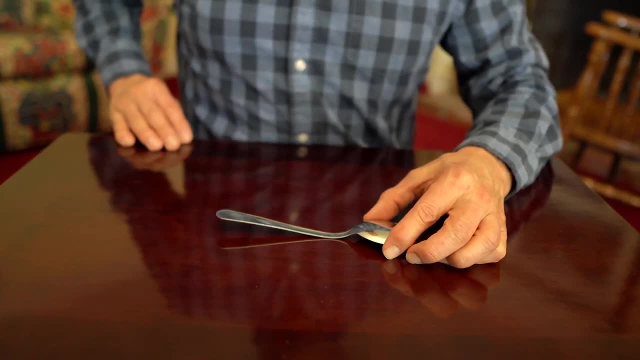 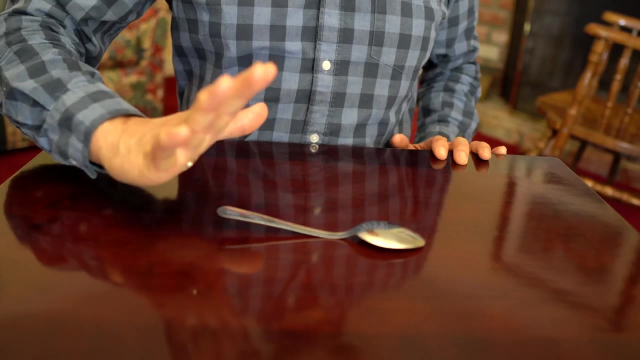 and stress-free, Then, by waving your hand, as it has, towards your back and you tuv this magnet on the table, Bring your spoon from over here and if you happen to be moving it by department o balm and kicking the hand at this way, it can bounce off the table. 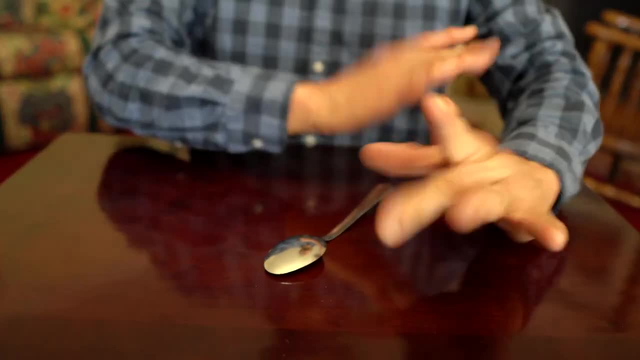 Make sure your hand is far away, depending on the strength of- and thenمر Filipom 대� caller pron. understand, by waving your hand here, you can capture the spoon and start causing it to spin as if you're moving it with your mind, and then you can. 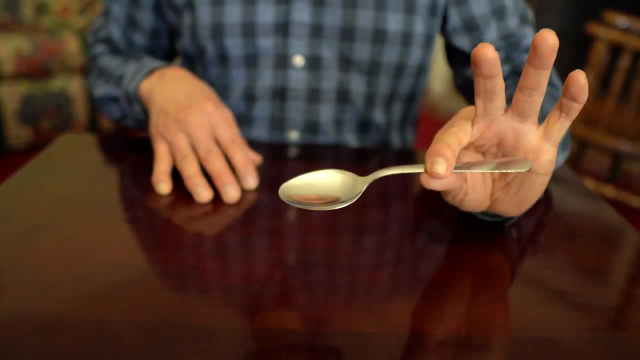 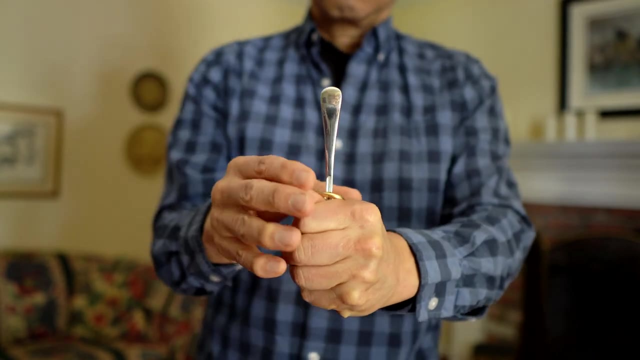 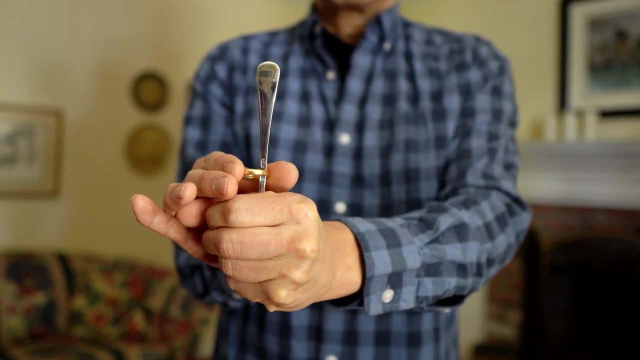 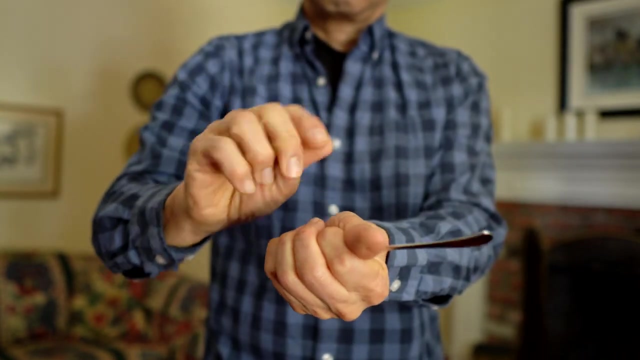 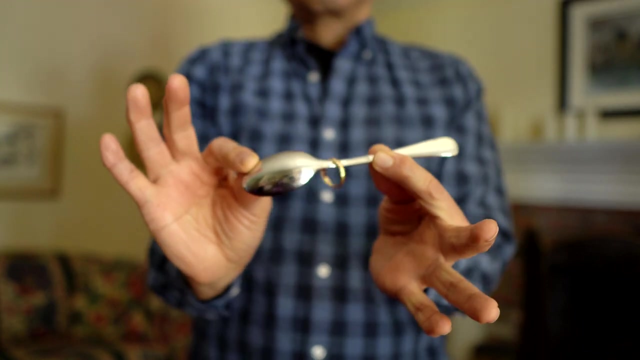 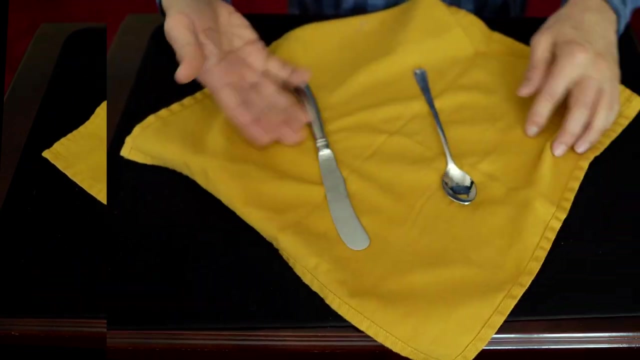 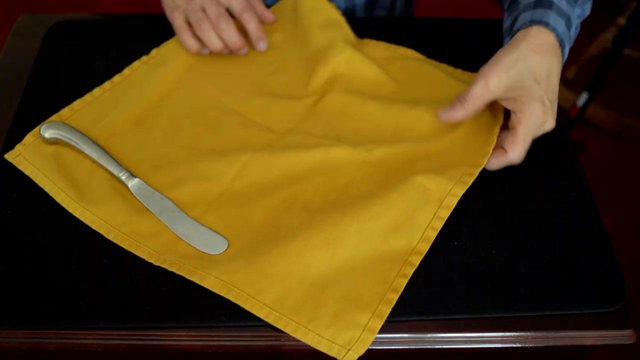 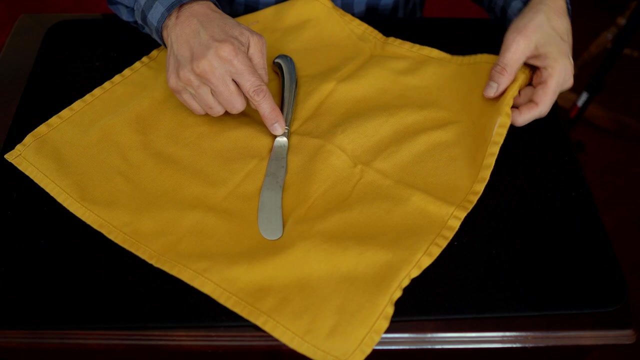 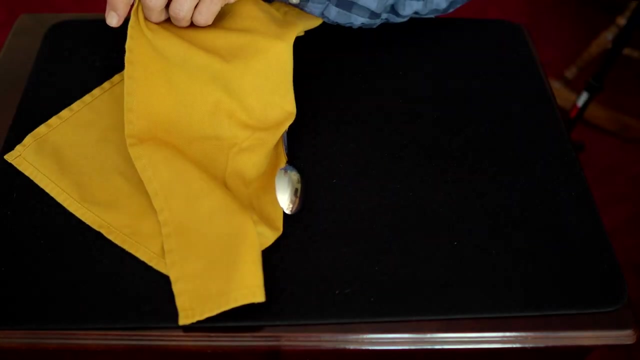 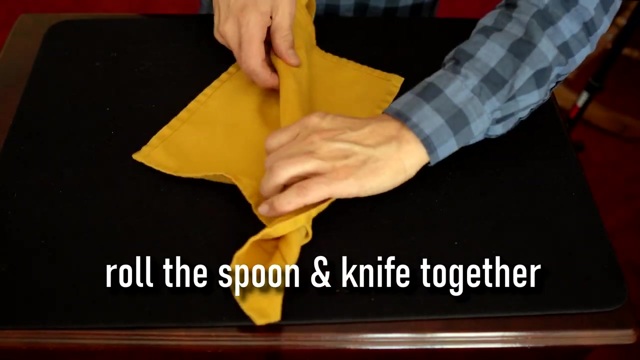 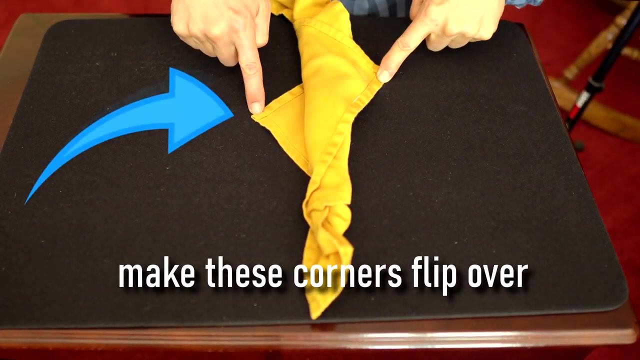 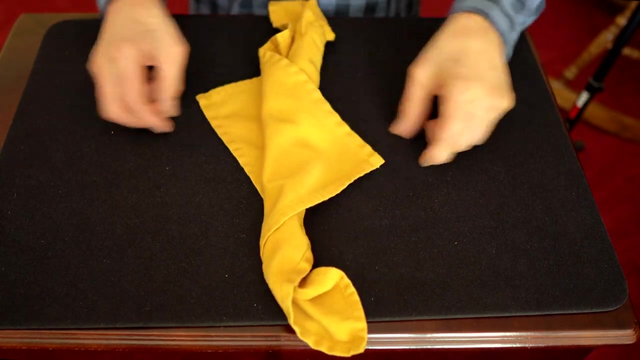 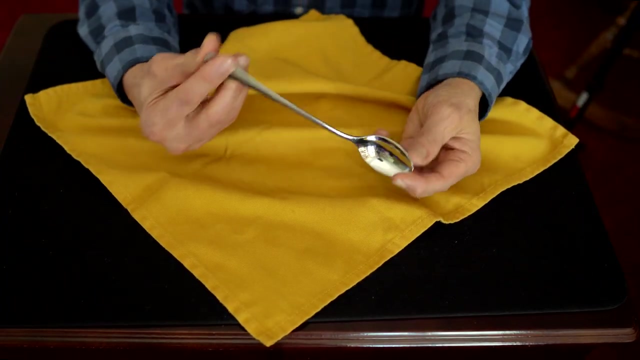 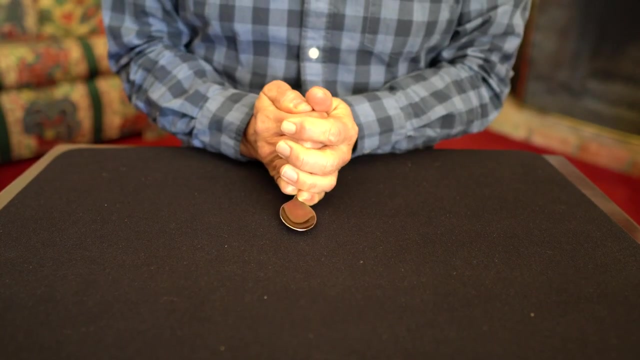 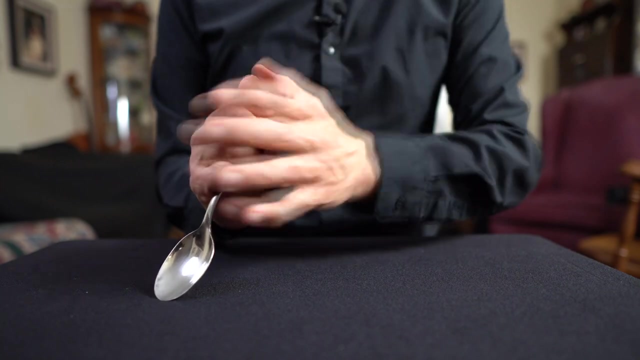 freely show the spoon at the end and have spectators examine it. Thank you for watching. Thank you for watching. All you need is an ordinary spoon and it's all in how you hold the hands. Now see, it looks as if I'm bending the spoon.